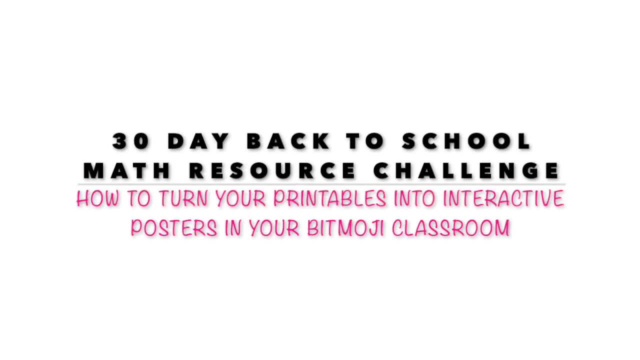 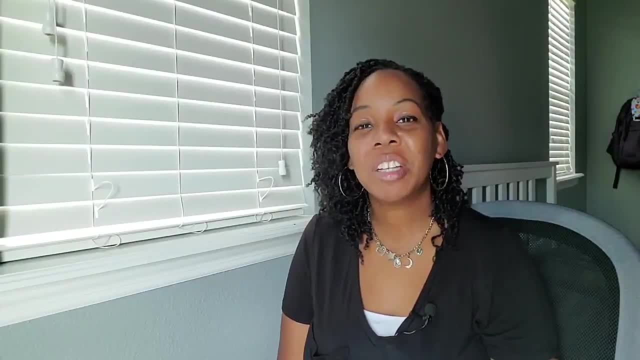 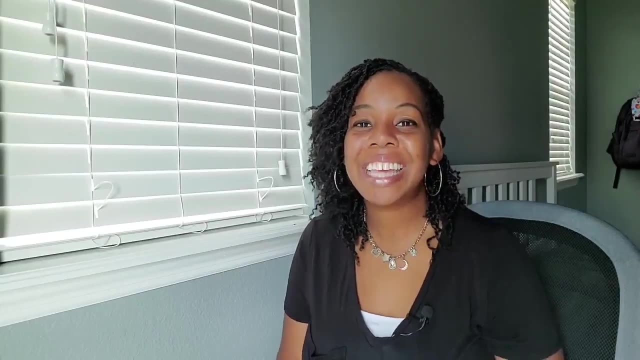 Hey everyone, welcome back to my channel, MathVal. My name is Michelle. Here I share strategies, tutorials, ideas, tips and more in elementary math for parents and teachers. Today is day seven of our 30-day back-to-school math resource challenge, And in today's video I'm going to 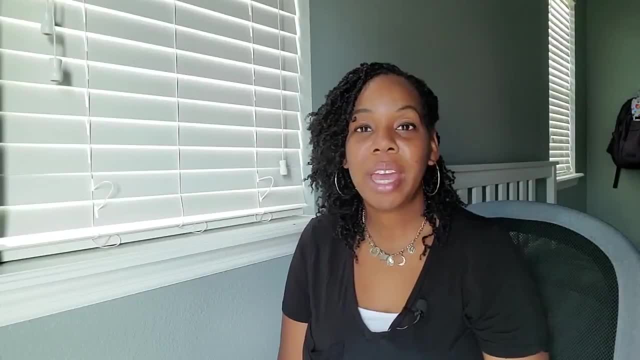 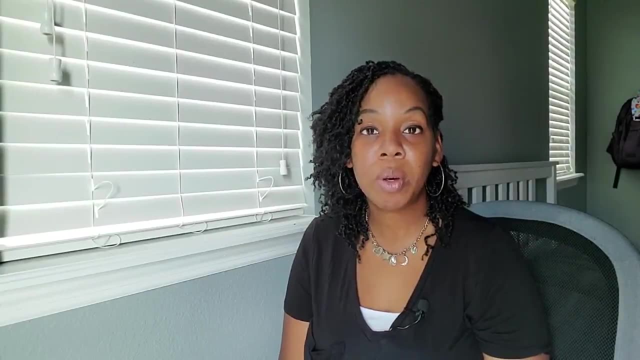 show you something a little different. I'm not going to show you how to create a printable, but actually a digital resource. Right now, a lot of schools and a lot of teachers are teaching remotely or using a digital distance learning platform, So I want to show you how to create. 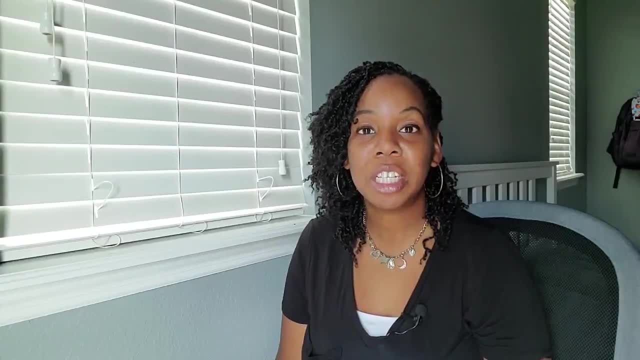 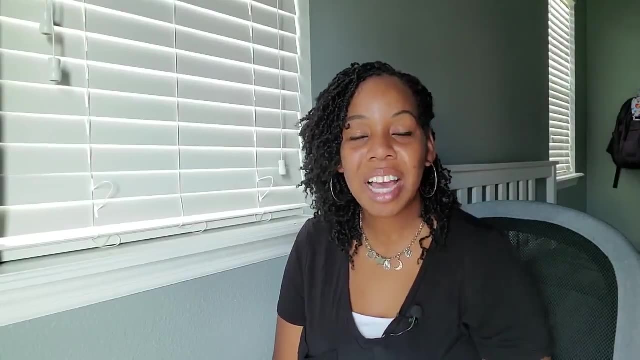 a visual, a digital visual, to add to your digital or virtual classroom. A lot of people are using bitmojis to represent them as the teacher in the classroom, And you can have so many different things in your virtual classroom. I want to show you how to take some of your PDFs. 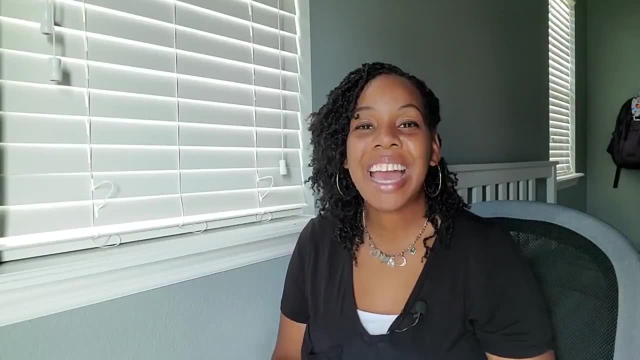 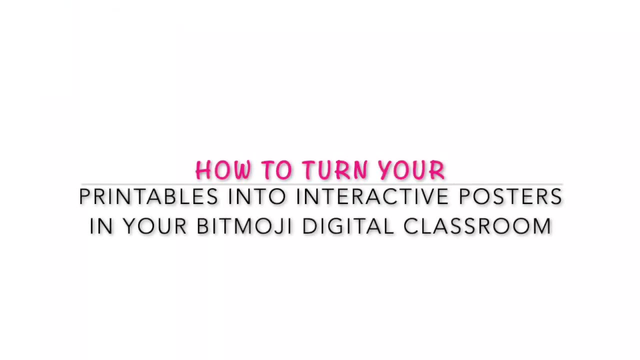 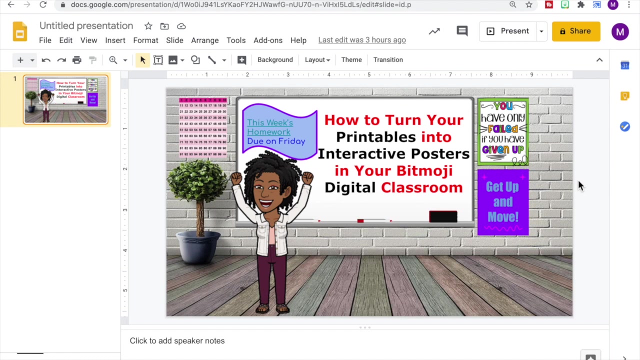 that you've created or you've purchased or downloaded and add them to your virtual classroom. Let's get started. I'm going to show you how to turn your printables into interactive posters in your bitmoji digital classroom. So if you want to create visuals or posters to have in, 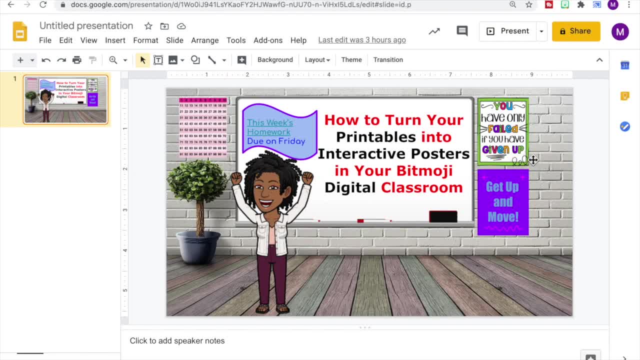 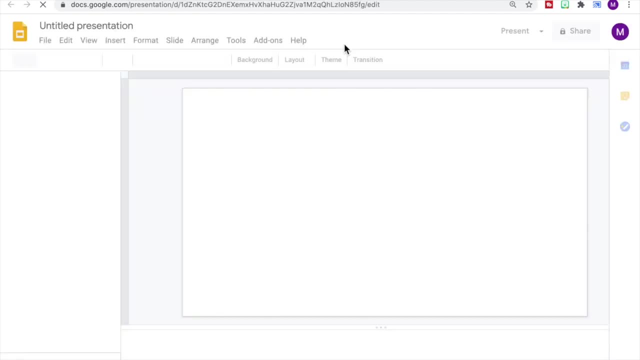 your digital classroom. I'm going to show you just that, And I'm going to be using Google Slides for that. So what you're going to want to do is start a new presentation. So we're going to go to File New Presentation And I'm just going to show you how to set up a basic bitmoji classroom or digital. 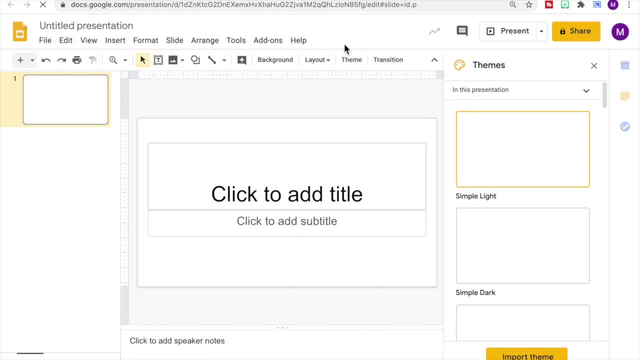 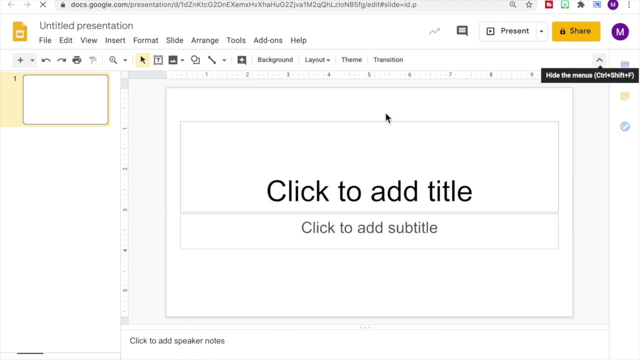 classroom. We're not going to add in too much. I just want the classroom set up And then I'm going to show you how to create those visuals or those posters. So let's X out of our themes, Let's change our layout to a blank slide. 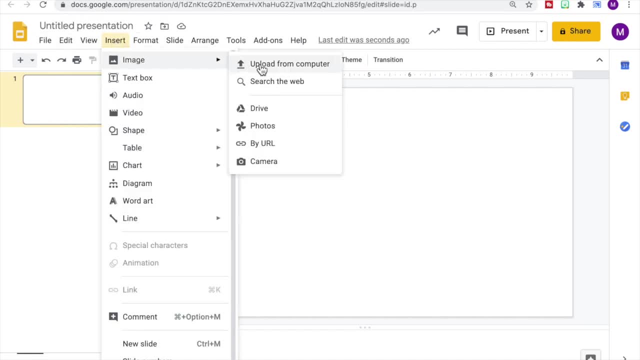 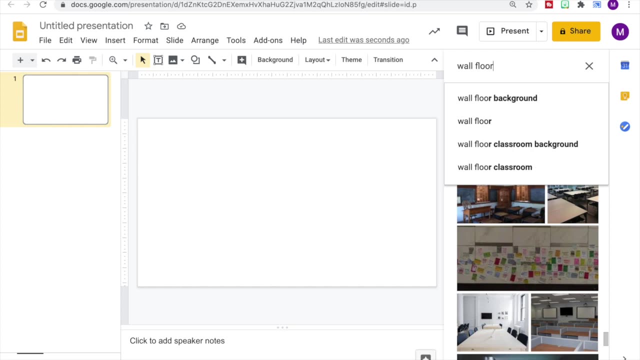 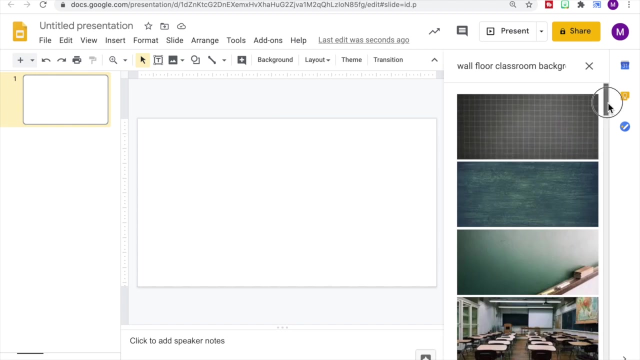 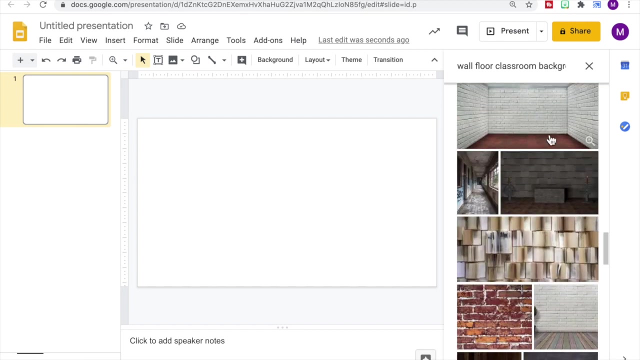 gonna go to insert image and search the web. I'm going to type in wall floor and then I see it says wall floor classroom background. so I'm going to click on that and see what they have. there's a. there's one that you can use for a virtual. 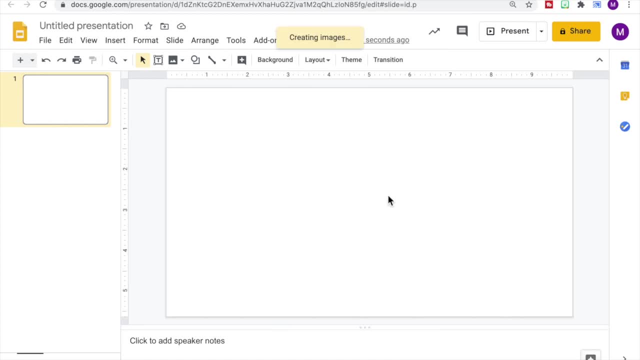 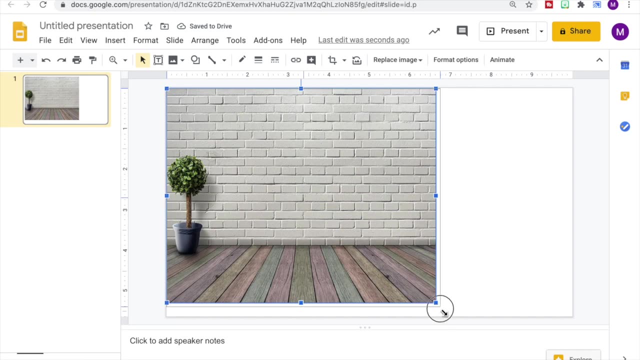 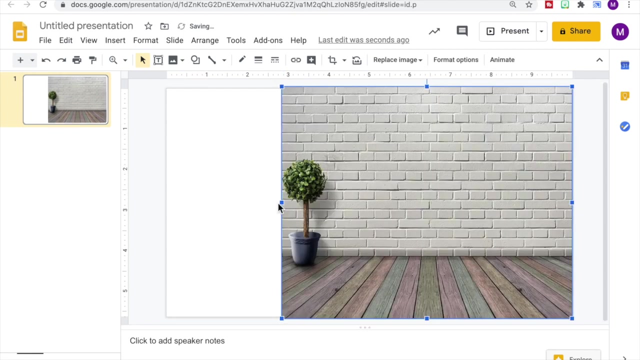 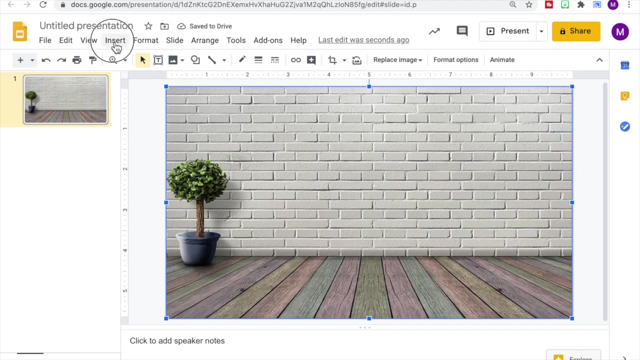 classroom, and here's the one that I want and I choose insert and then just stretch it out to cover the entire slide. so there's our background. so the next thing I want to do is insert like a whiteboard. so I'm going to go back to insert and 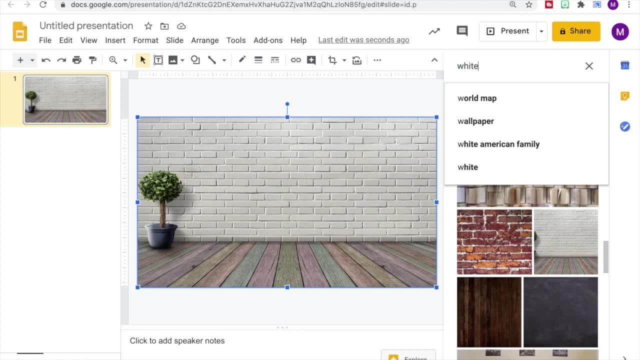 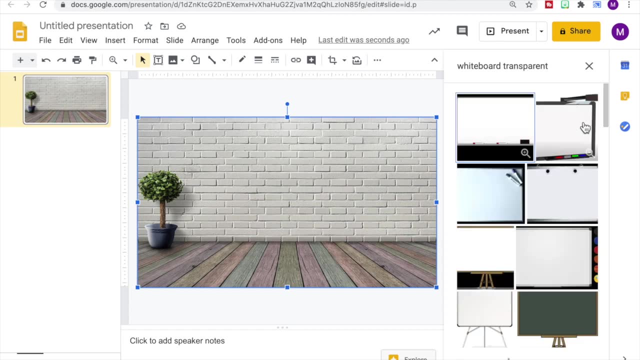 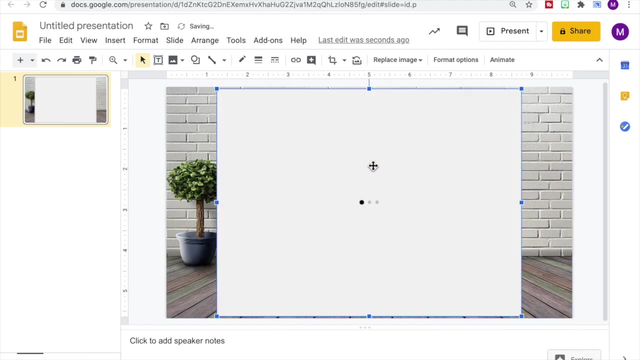 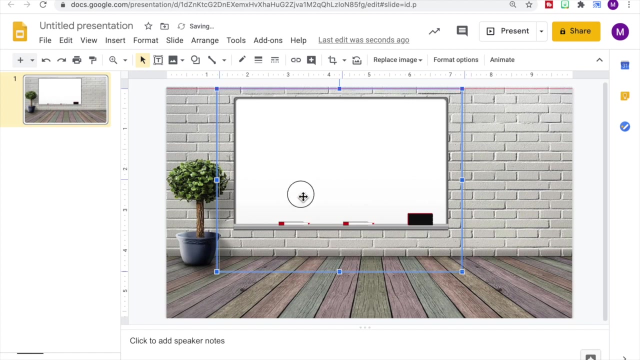 search for the background, and then I'm going to click on that and then I'm going to search the web. I'm going to type in white board, transparent, because I don't want it to have a white background with it. let's try this first one insert and that is the one I want. so I'm going to resize it. 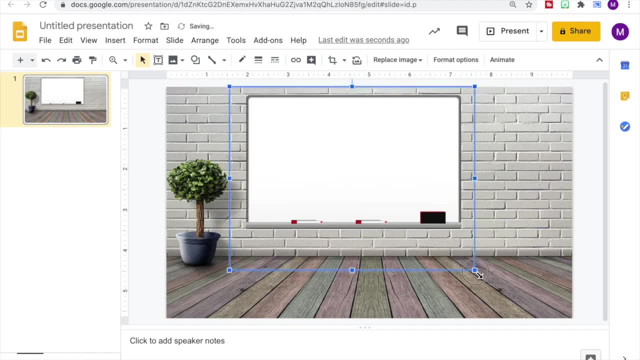 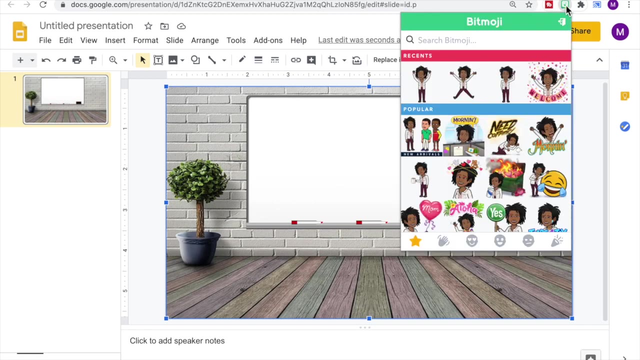 and just move it over slightly. so there's the while I'm going to add this. So there's a basic setup that I want. of course you can add in a desk, a table, different shelves, but here's our basic background- And then adding in a Bitmoji. you need to download the app on your smartphone and then 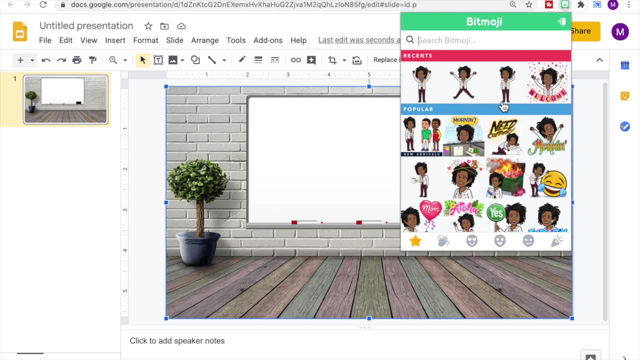 add the Chrome extension onto your computer and then you'll have access to your Bitmoji where you can insert them. So you can do this now, or you can do this towards the end, after you've added in your posters or your visual aids. I'm going to right click one of my poses, copy image, and then click here and click paste. 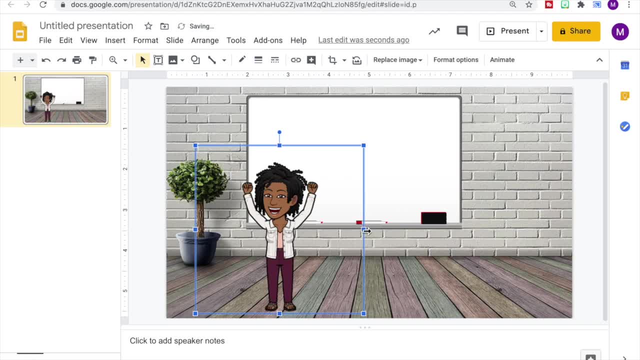 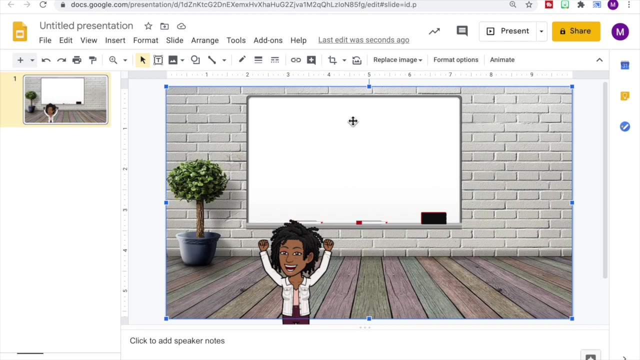 And there's my Bitmoji. I'm just going to move her off to the side for now, towards the bottom. So now I want to add in some posters or visuals for the students to see, So you can create your own. you can use ones that you purchased or ones that you found. 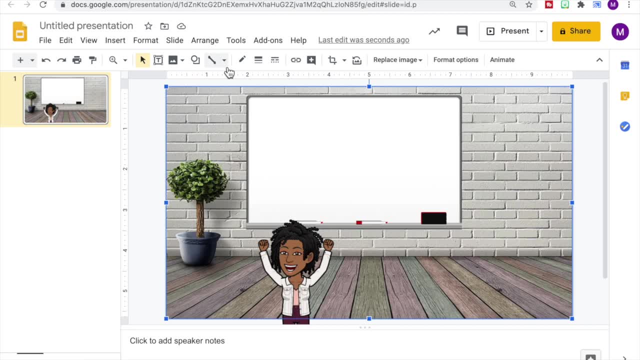 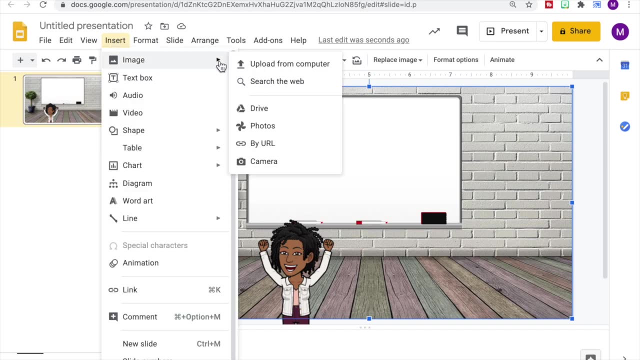 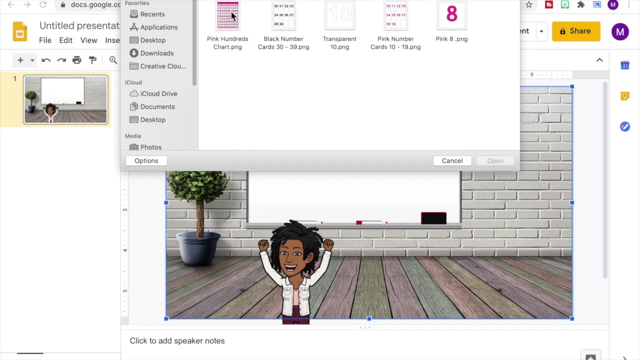 online. You can use them for free. So what I'm going to do is add in one of my printables that I've created a hundreds chart. So I'm going to go to insert image and then upload from computer. So here's the chart that I want to use. 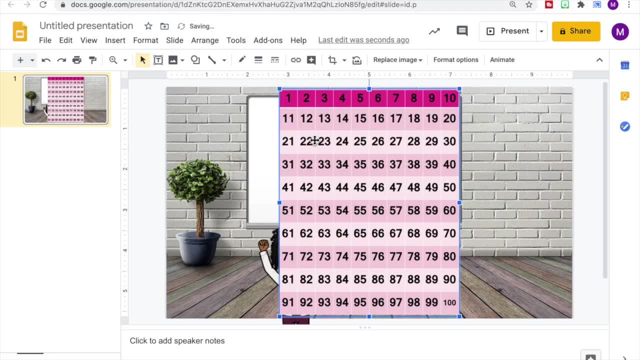 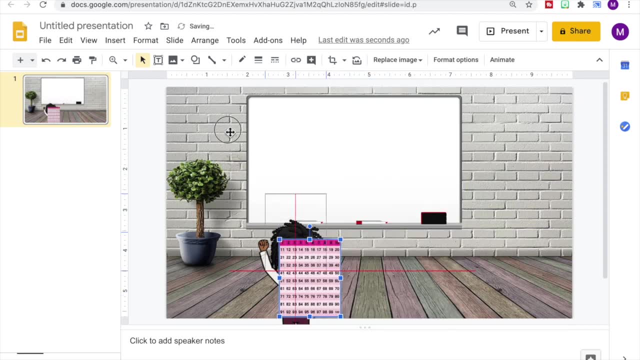 It is an image, it's a PNG, so I'm just going to double click on it and it pops right into my scene: my digital classroom. So I'm going to minimize to fit the background, So I'm just going to double click on it and it pops right into my scene: my digital classroom. 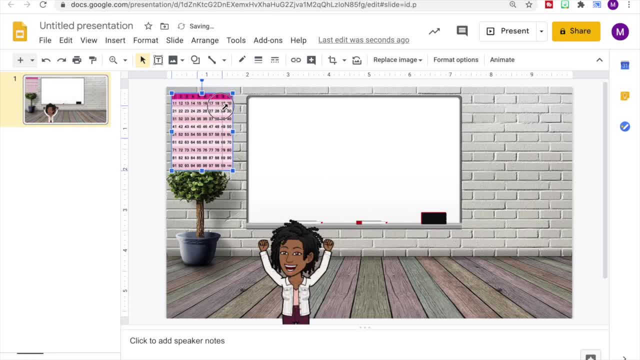 So I'm going to minimize to fit the background. So here's the chart that I want to use. I'm just going to double click on it and it pops right into my scene- my digital classroom. So here's the chart that I want to use. 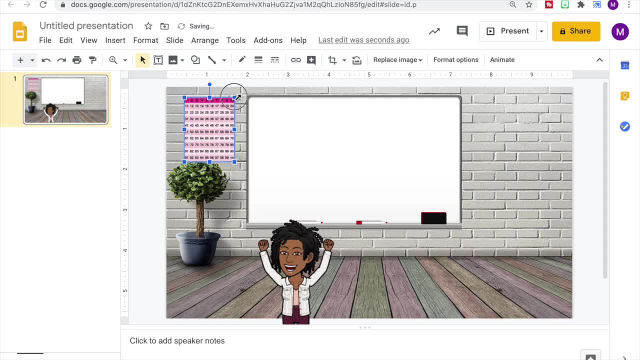 It is an image, it's a PNG, so I'm just going to double click on it and it pops right into my scene, my digital classroom. You can pretty much place it wherever you want. I'm just going to put it back here and then I'm going to add a link. 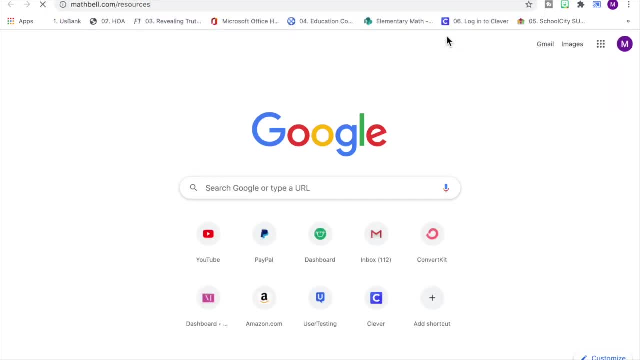 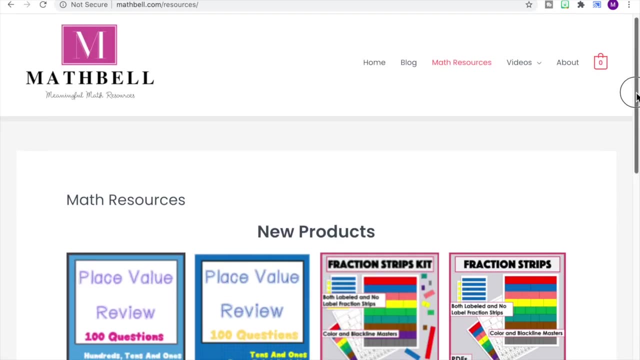 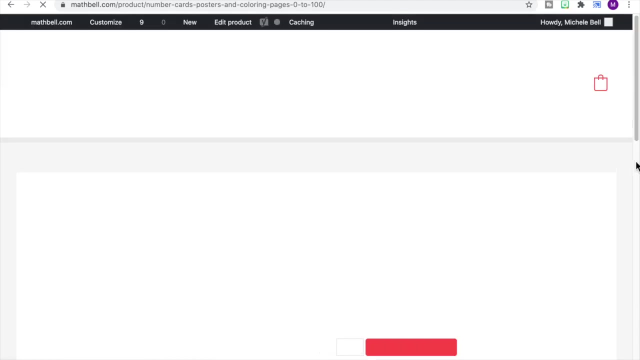 So I'm going to go to mathbellcom slash resources to find where I can access those hundreds charts, And this is just doing this for the purpose of this tutorial. Um, of course, for your students, students, you don't want them to have to purchase any products unless you're. 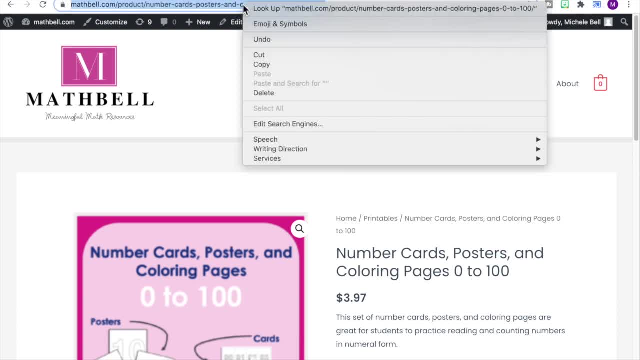 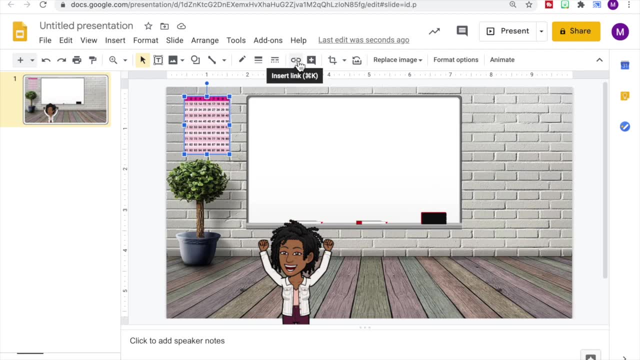 sharing it with families for them to purchase. so I'm gonna copy this link and then go back to my presentation. when I click on here, then go up here to insert link, right click and then hit paste and then apply, and now that link is attached to that image. so let's insert a poster or a document from something that you 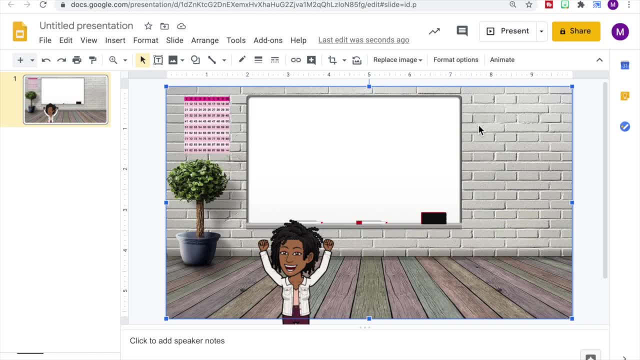 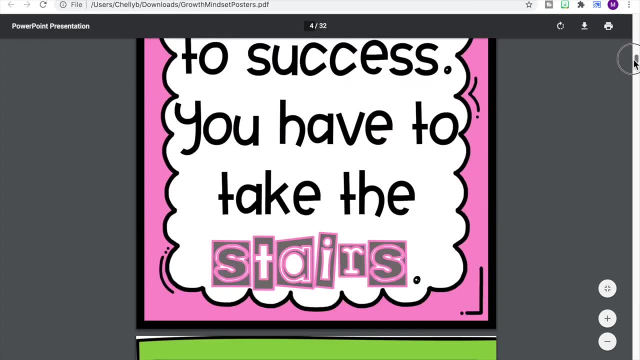 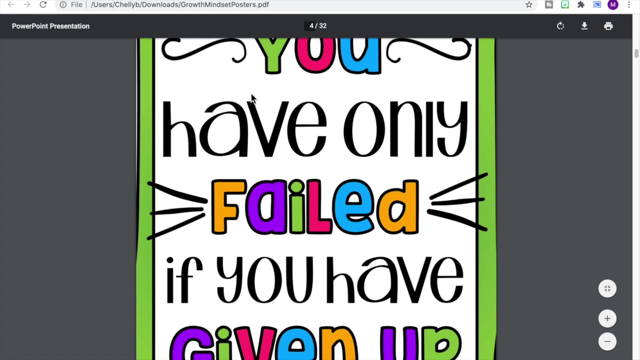 maybe found on teachers pay teachers or Amazon, or you've downloaded or someone sent you. so I have these growth mindset posters that I got on teachers pay teachers and a one of them I took a screenshot of to get an image and picked it up earlier and went over it and then, like I just want to go ahead and 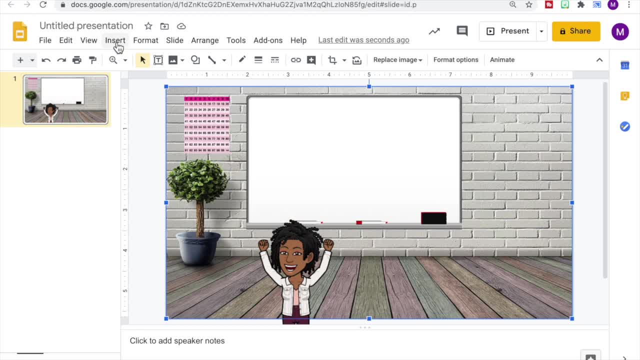 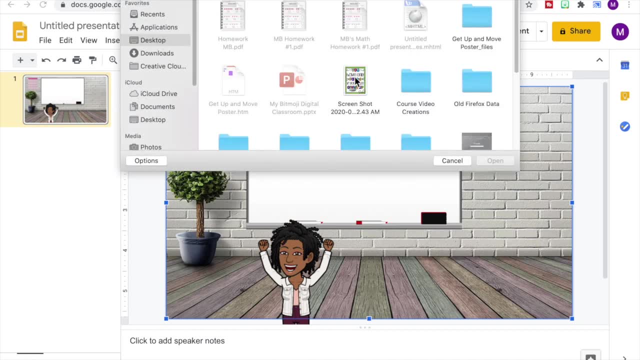 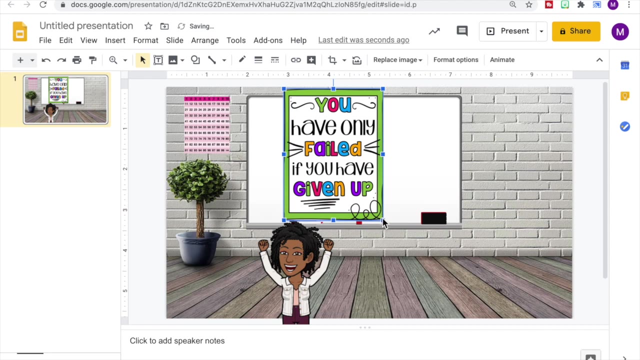 And I'm going to insert that into my page. So I'm going to go back to insert, go to image upload from computer and then go to my desktop and then find that image, that screenshot, double click it and then resize it. 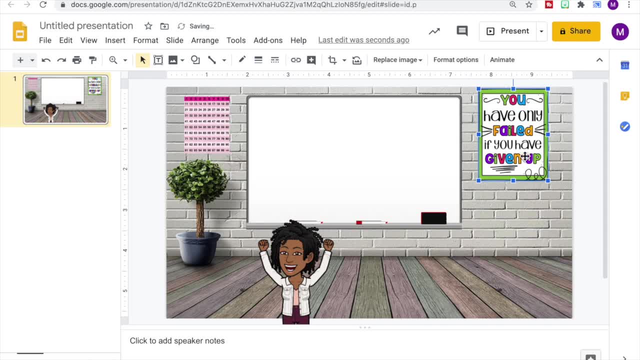 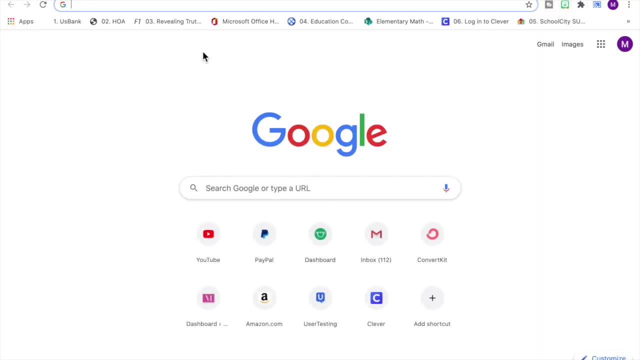 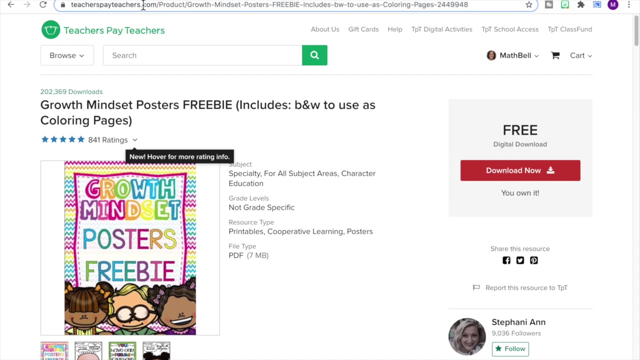 Let's make it a little bit smaller. And then I'm going to link that one to the store on Teachers Pay Teachers that I found that item. So here's the page of the posters that I have and the author that created them. She did such an awesome job. 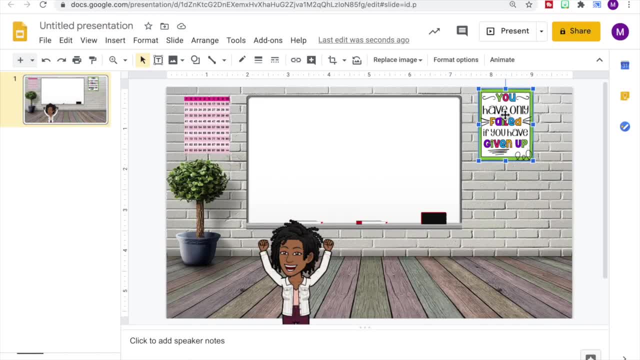 So I'm going to copy that link, Go back to my page, click on the image, go to link and then press paste and apply. So now that link is attached to that image. So what if you wanted to create your own visual? that there's not something out there that? 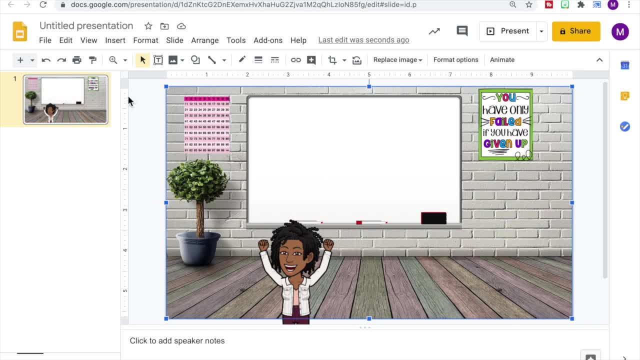 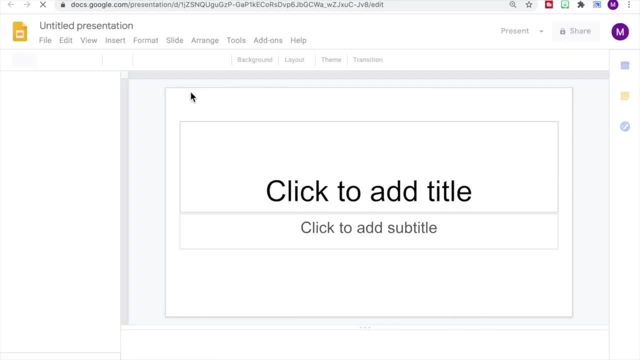 you like, but you wanted to create something specific for your students. So we're going to do that by starting a new presentation, And it's because I want to. I'm going to resize the slide size. I want it to be eight and a half by 11, so I need a new presentation. 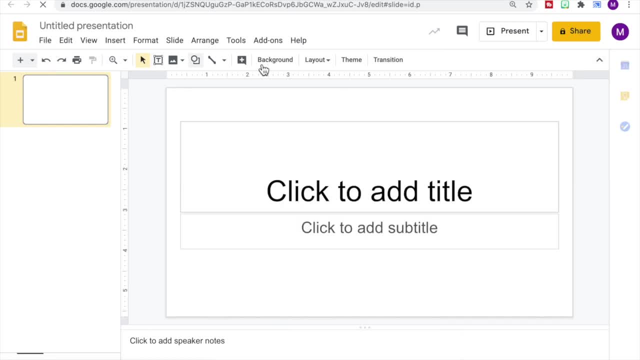 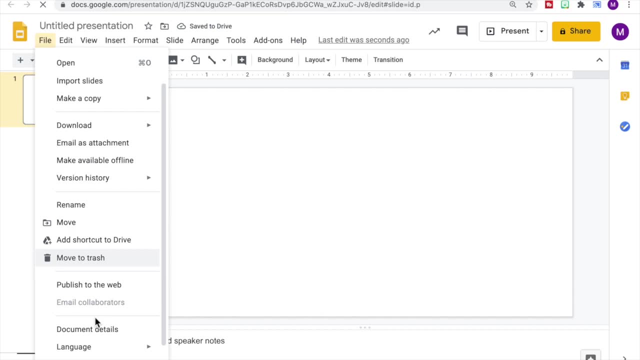 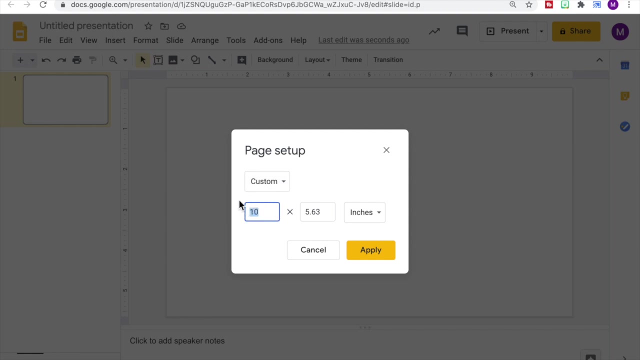 So I'm going to get rid of the theme. I'm going to change the layout so I have a blank slide. I'm going to go to file and go down to page setup and then click on the drop down menu, hit custom and then change the dimensions to eight and a half inches by 11 inches and 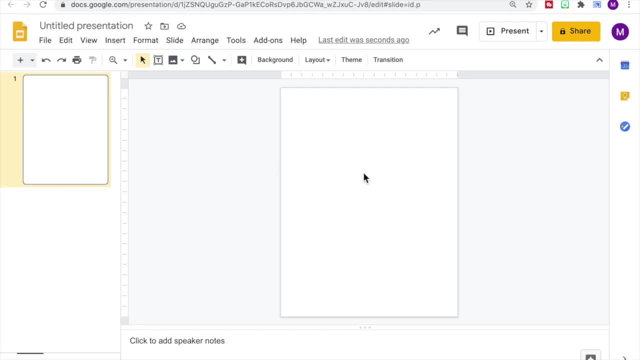 hit apply. So now we have our blank canvas. that's eight and a half by 11 inches. So now I want to create just a visual So my students are going to stop and do some kind of movement or activity, And maybe I want to link it to a YouTube video. 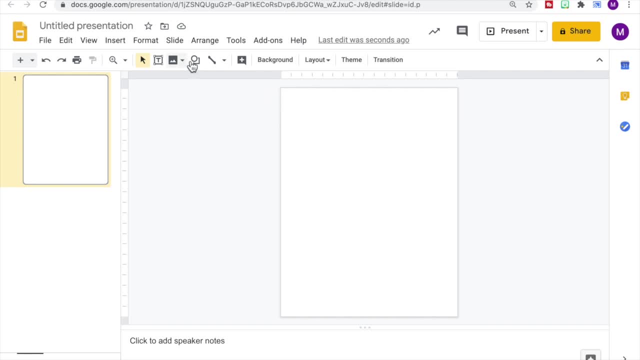 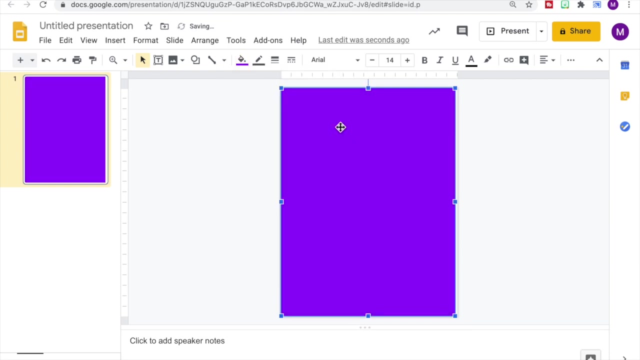 I just want to create a visual for that. So what I'm going to do is add a shape so I can have a background. Okay, Okay, Okay, And I'm gonna go up here to fill color and choose the color that I want. 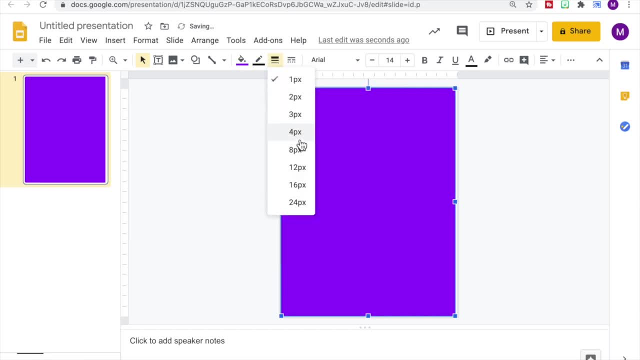 And the border. I'm gonna choose black. The thickness of the border, let's choose four, Let's choose eight, And then let's make it dotted. So now I'm just gonna type inside, I'm gonna type, get up and move. exclamation point. 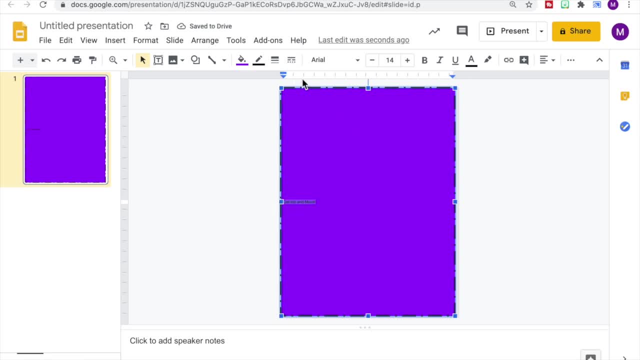 So now the text is really small, So we need to increase that text. Let's center it first, Then let's change the font, Let's go with impact, Then I'm gonna hit the drop down on the font size and go as large as I can go. 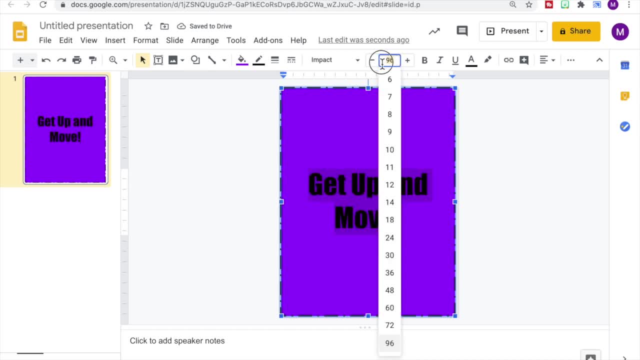 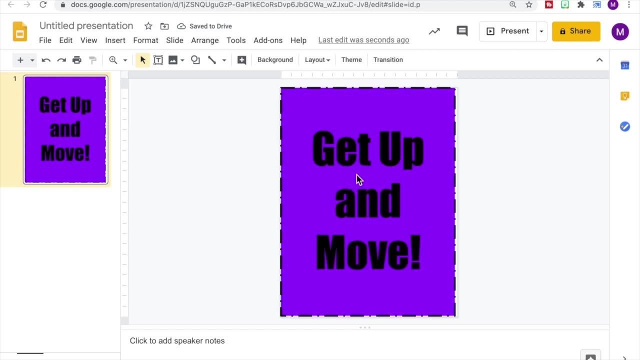 Still not large enough. So I'm gonna click into the font size and I'm gonna type in 150 and see what that does. So I like that size. Let's change the color. I'm gonna go to the text color and choose like a light blue. 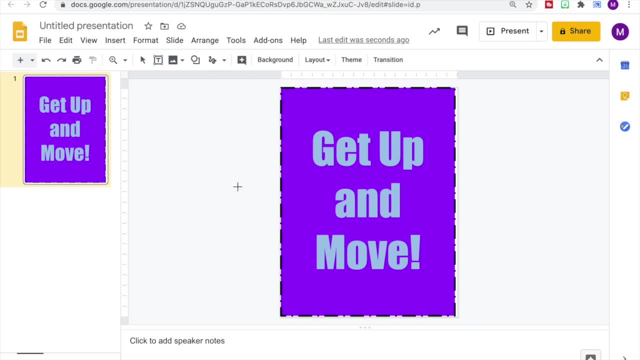 I like that. We can add in some design. I can add in this scribble, freehand scribble. It's not perfect but I like it. And then I'm gonna click on that and hit the line color. Let's change it to like a pink and make the size larger. 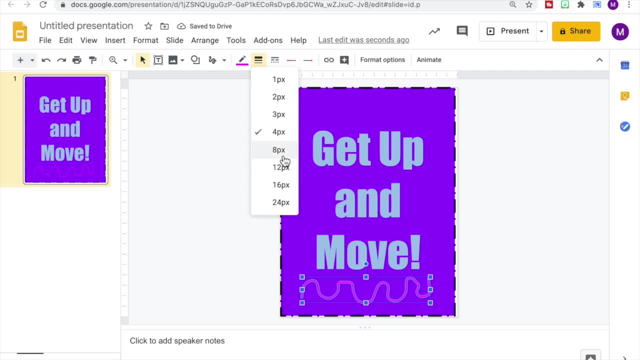 Let's make it thicker than that. Let's go with eight And then just to add some more pops of color. I'm gonna go back to shape and go to this call out section and click on like this star here: Select that. Select fill color. 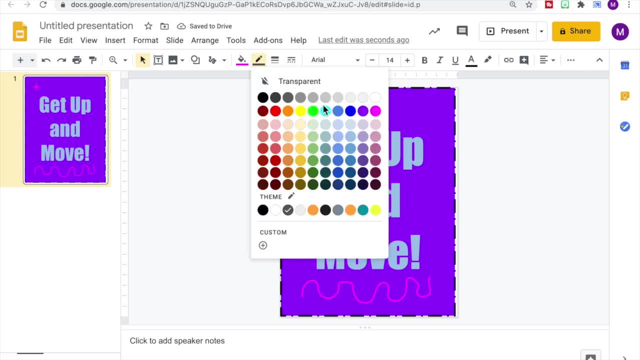 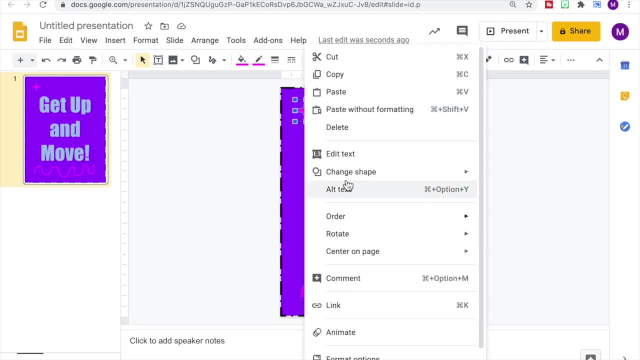 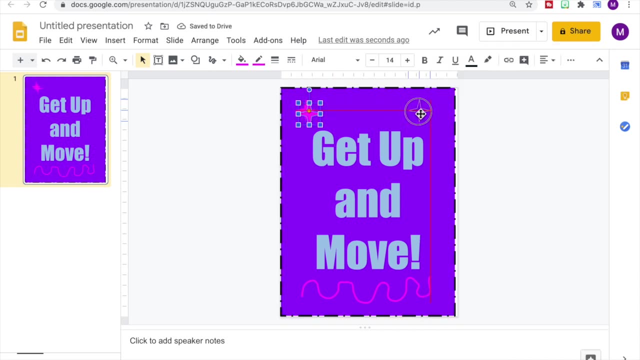 Go to pink, Change the line to pink as well, And then I'm gonna click on it, right click on it and hit copy, And then over here I'm gonna hit paste. Let's move that over. You could also have done duplicate. 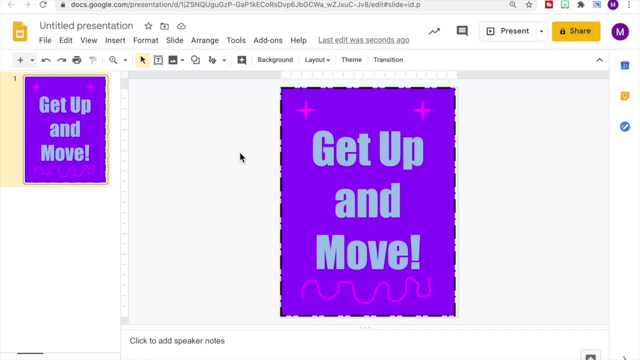 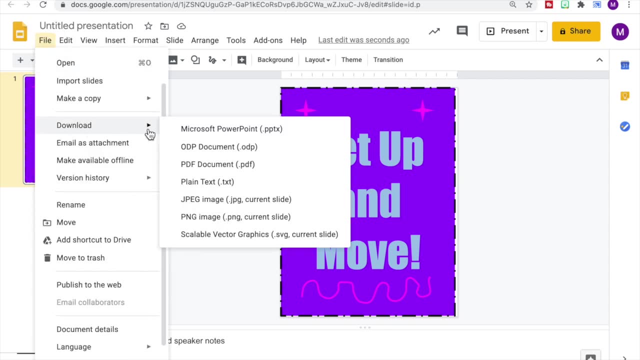 So that's just some pops of color that I like. So now I want to save this as a picture. So I'm gonna save the slide, I'm gonna go to file, I'm gonna go to download and then download as a PNG. 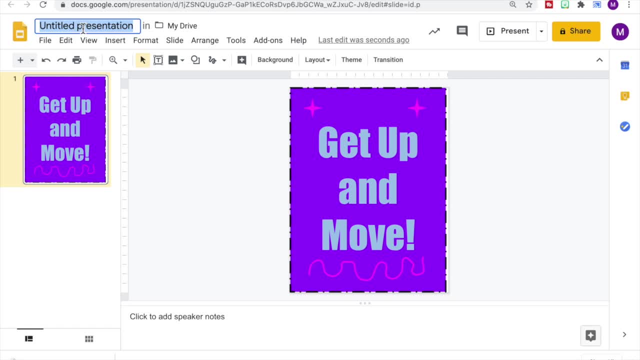 Oh, let me go up and give it a title. So I'm gonna put: get up and move poster. So now let's do that again. File download as a PNG. And now it downloads. If you click on that, there is our image. 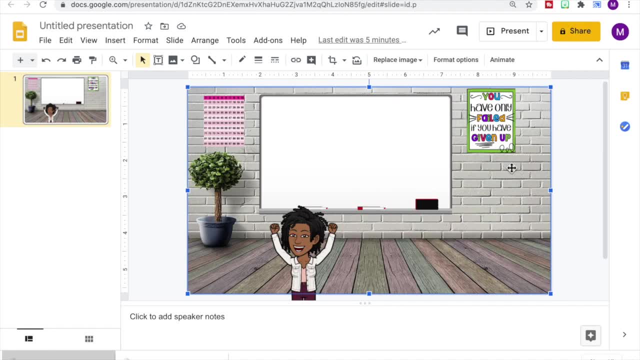 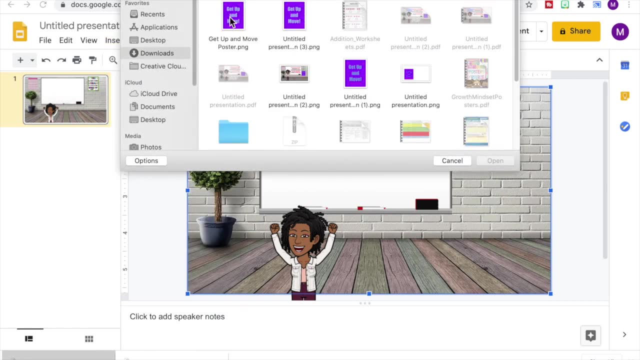 So let's go back to our digital classroom. I'm gonna go to insert image upload And then I'm gonna click on download from computer and click on my downloads and there is my poster that I just created. So let's minimize that. 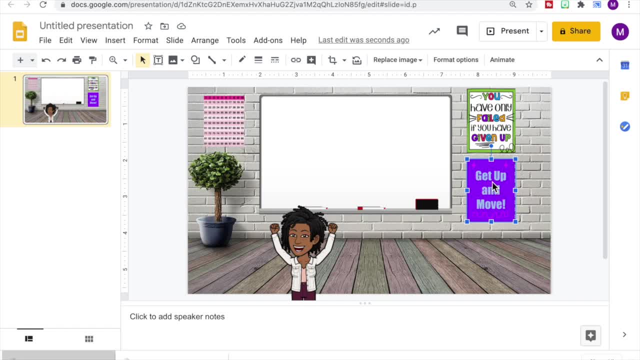 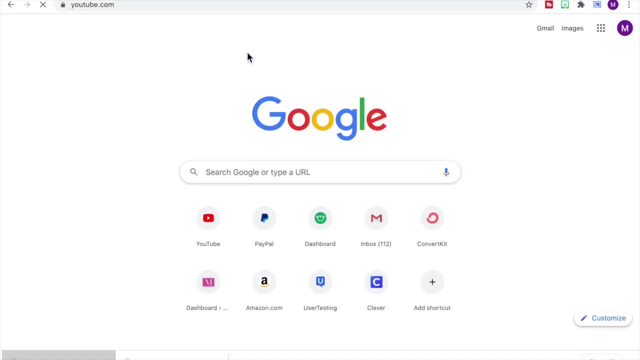 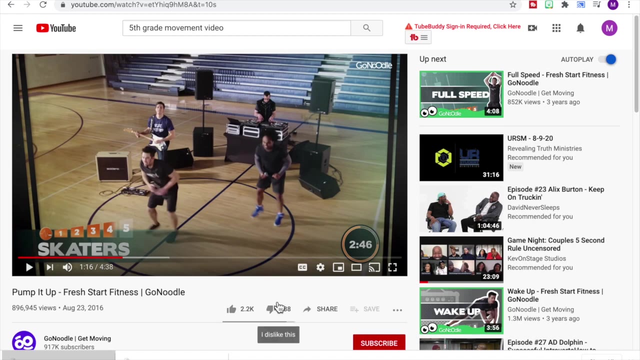 Okay, so now let's make it interactive. So we have get up and move. I'm gonna go over to youtubecom and I want to find like a video that the students can watch and move to. I found this video that I want to use for my students on youtube. 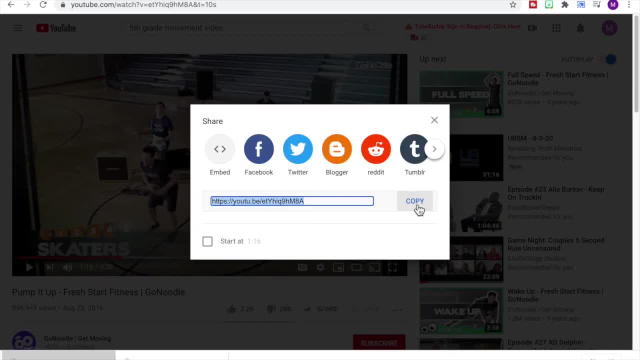 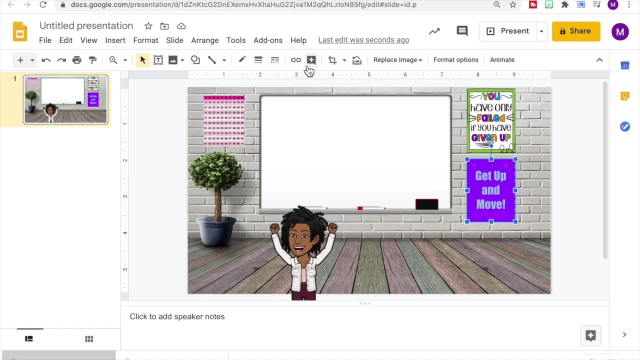 So I'm gonna go to share and then click copy and go back to my digital classroom. Click on that poster, go back to insert link, right click, then paste apply. So now that poster is interactive, We click on it, It's gonna link right out to that youtube page. 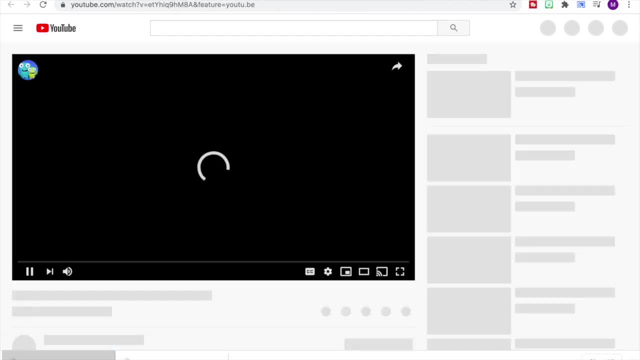 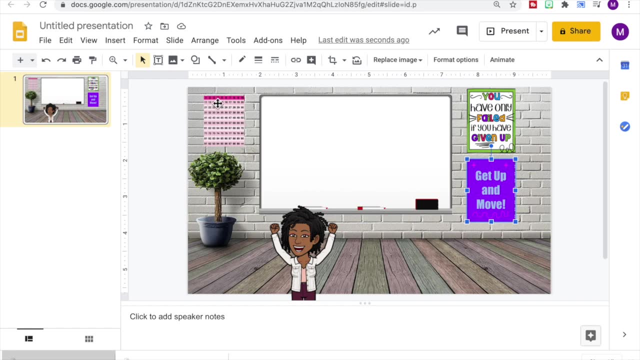 so that students can watch that video, that video. So now it's linked to the video and the students can watch it. So we have three different visuals. Let's add in one more way to make our posters, our visuals, interactive. So I'm 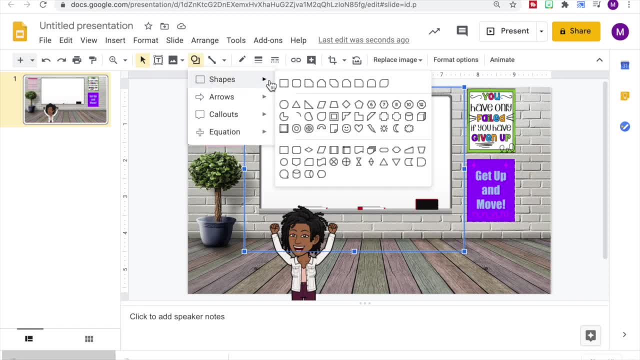 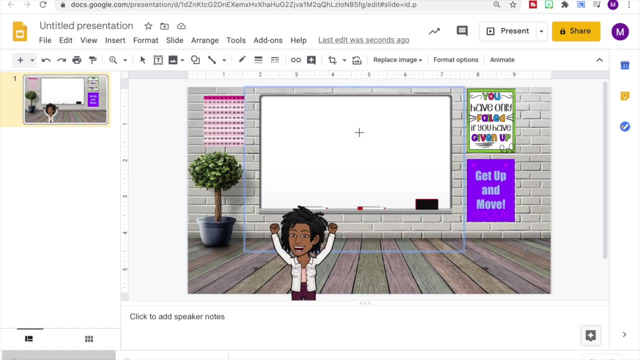 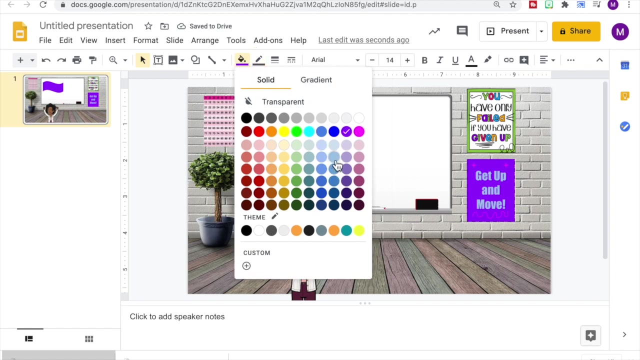 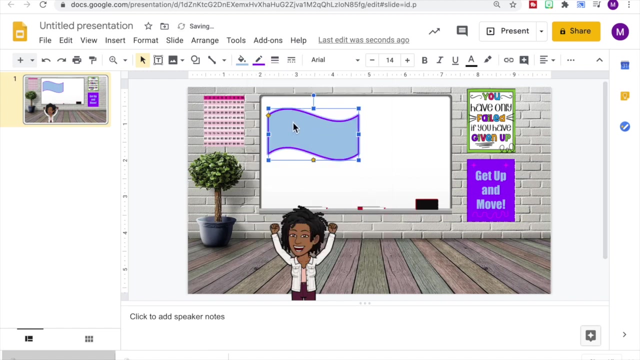 going to add a shape. Let's add in, let's change our background color, Let's make this a purple and our actually let's make it blue and make our line purple and our line a little thicker. And then I'm going to type inside um weekly homework assignment And then I'm going to put 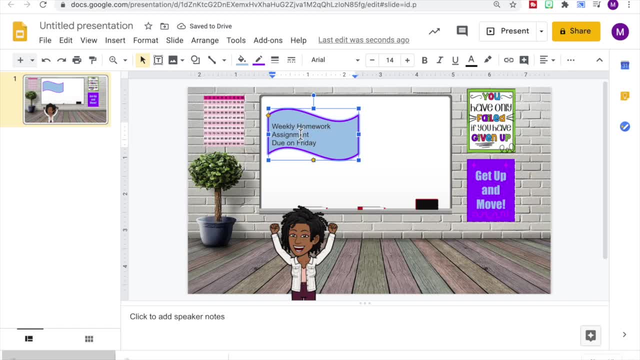 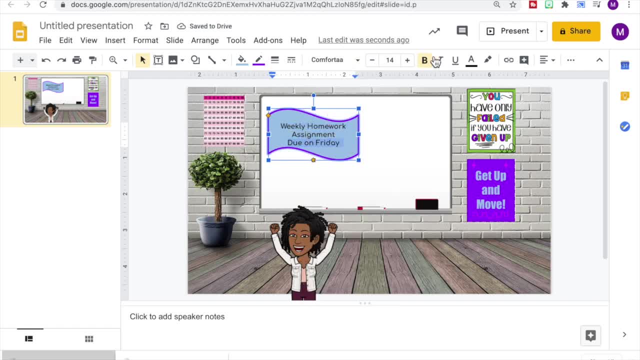 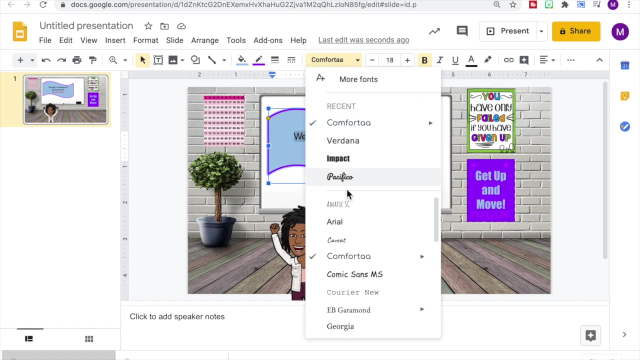 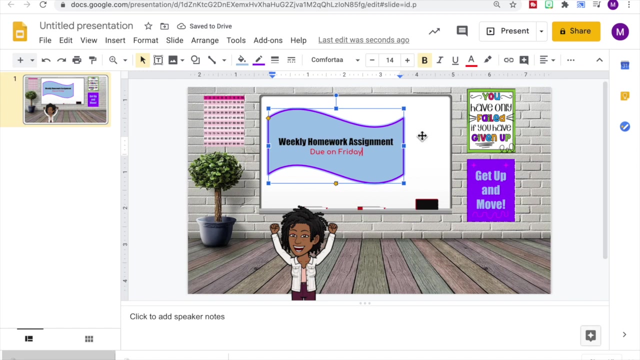 change the font. Let's make the due on Friday. Let's put that in red and let's make our weekly homework assignment a little larger. Let's stretch out our shape, Okay. So there is our weekly homework assignment, like announcement or alert or something like a. 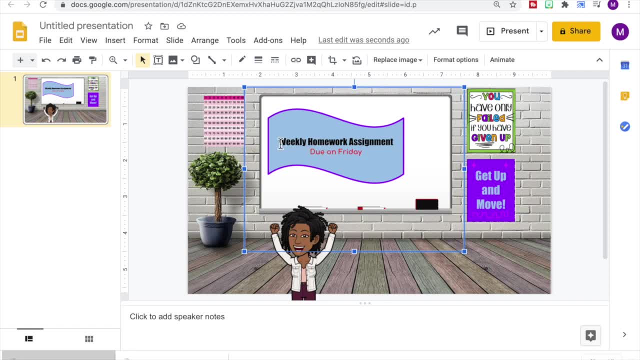 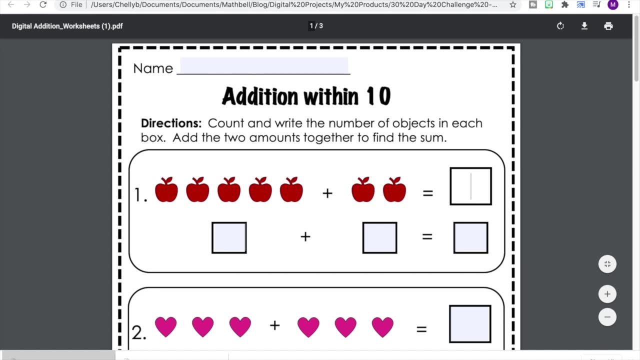 bulletin. So now I want to link it to whatever, whatever assignment that I'm going to give the students. So I'm going to find the page that I want them to work on. So I have this page that I actually created in one of the other videos for the 30 day challenge. just creating your own. 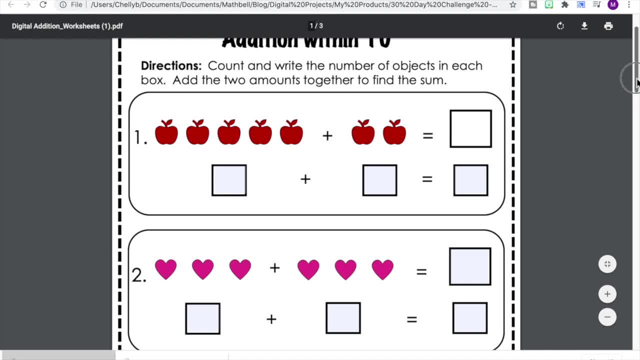 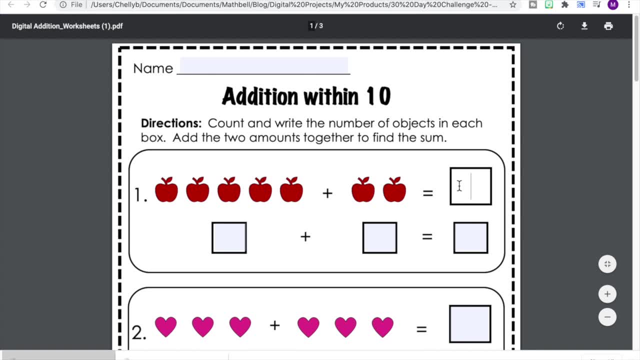 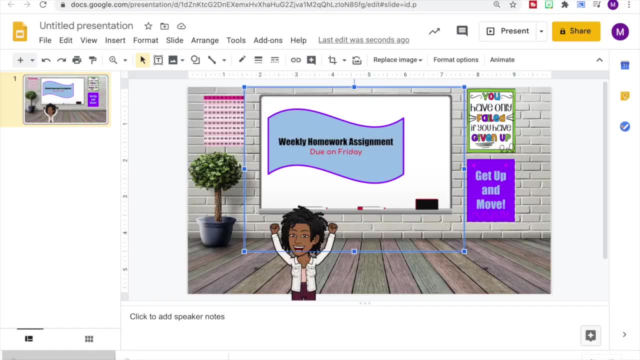 edition worksheets And I used the website PDF escapes to make it digital So students can type in their answers and save it and email it to you when they're done with it. So I'm going to take the link from this page and copy it, go back to our digital classroom And I'm going to select the text that I want to be. 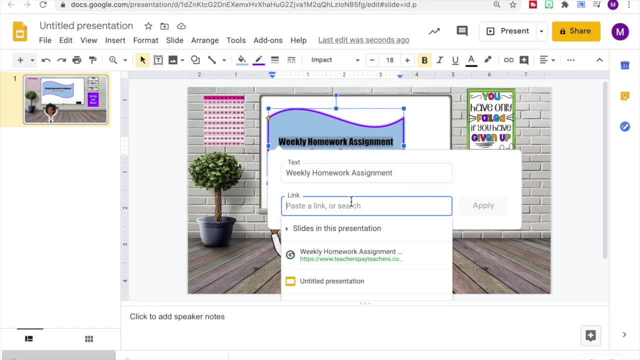 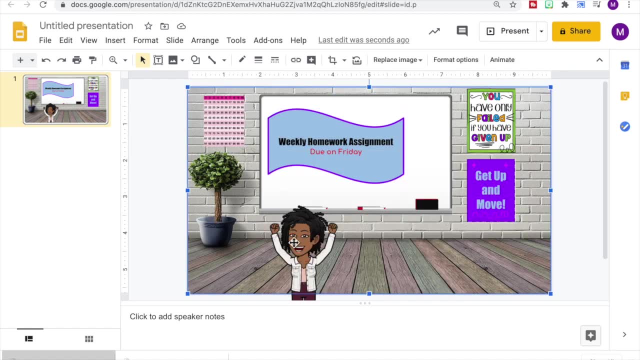 hyperlinked, go over to insert link right click, paste and apply. So now that is complete. So now I can add back in my bitmoji: Let's bring it to the front. Let's change the order and bring to front, Make it a little larger. So yes, I am excited about my digital. 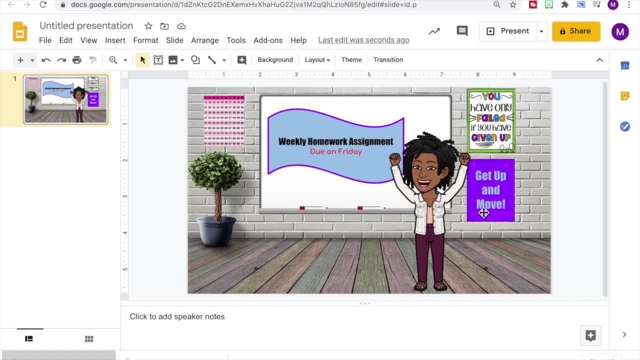 classroom. It's not complete because I want to add in more features, But I just wanted to show you how you can add in these visuals, these posters, and make them interactive for your students. So what I'm going to do now is: let's change. 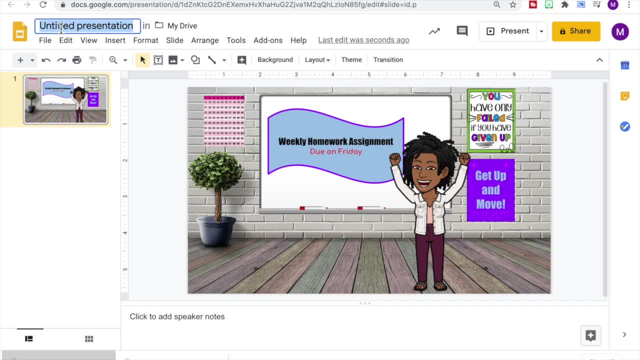 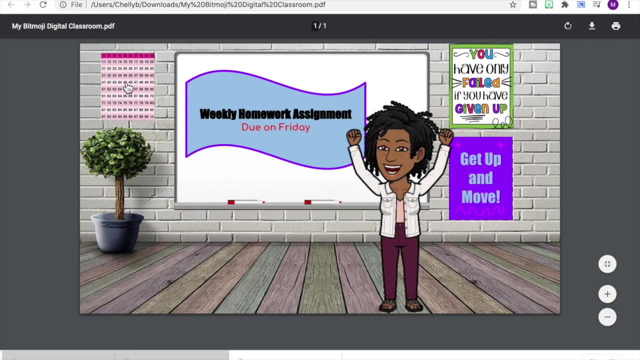 let's save it and give it a title: My bitmoji digital classroom. And then I'm going to go to file download And this time I'm going to download as a PDF document. So now it has been downloaded And if you just hover over those visuals, you can see that you can click on the different 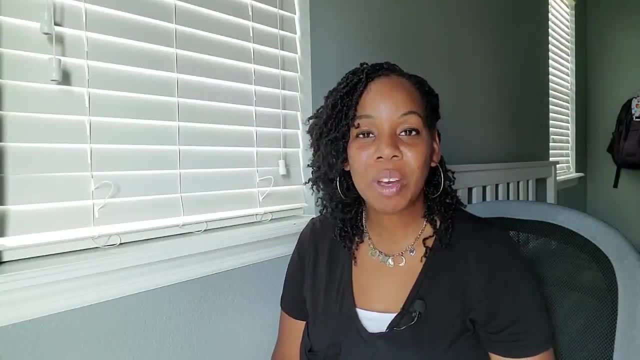 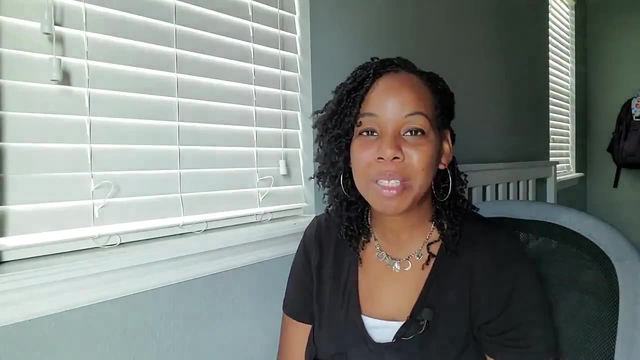 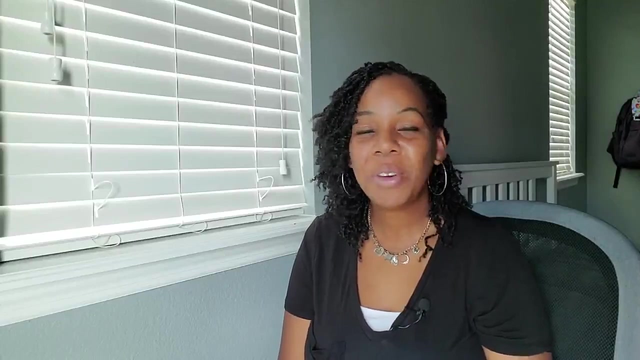 items. So that's the end of day seven. I hope you enjoyed that tutorial on how to create visuals for your digital classroom. Please remember to like, share and subscribe to my channel, And if you want to be notified the next time a video is posted, please hit that notification bell. See you in the 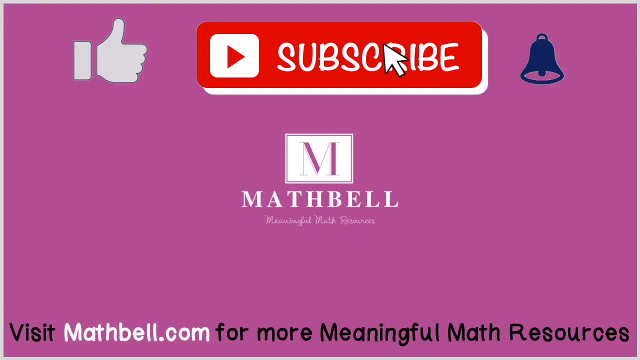 next video. Thank you for watching.